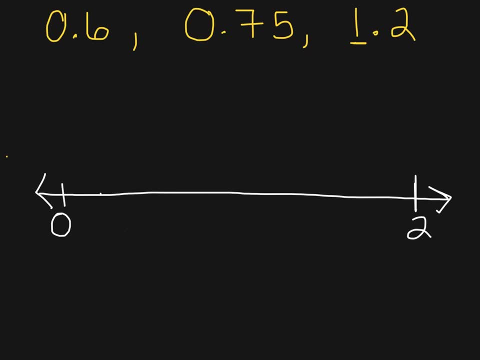 it's not fun to jump by twos when we're putting numbers on a number line and we know that halfway between zero and two is the number one. So in between zero and two, about halfway place a number one- Awesome. Let's actually put these numbers on our number line now and let's start with six. 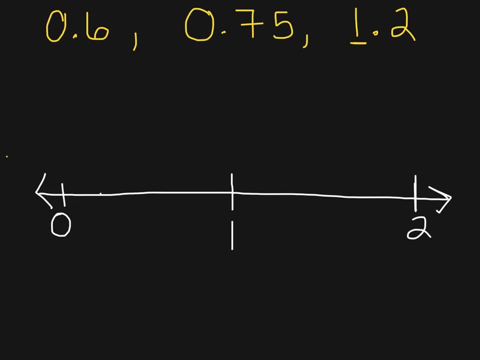 tenths For six tenths. that means that we need ten spaces between the zero and the one, because ten tenths make up one whole All right, and so the tenths place in the decimal is kind of a giveaway to how many spaces we need. 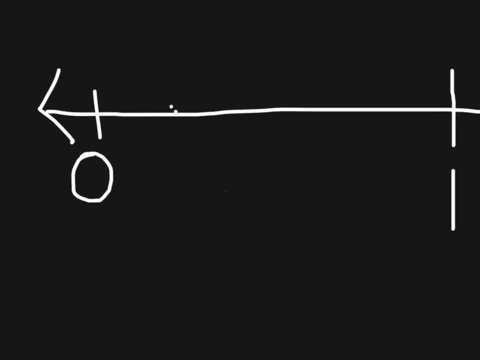 between zero and one. So let's zoom in between our zero and one and remind ourselves that we're working with the number six tenths, and since we need ten equal spaces, I kind of like to have a halfway point first, just like we did the halfway point between zero and two. So halfway between. 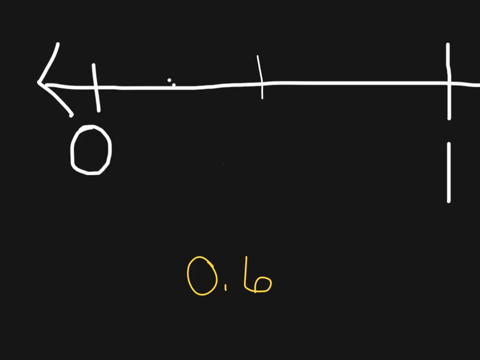 zero and one is the number. there's half or five tenths, So we already have half of our work cut out for us here. Now our next thing is we need to figure out how are we going to make equally spaced lines between the zero and five tenths, and how many of them Reminder that we have to go by. 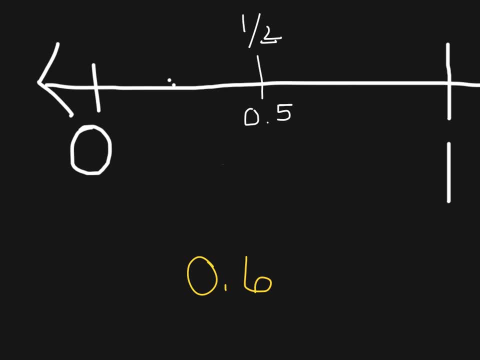 tenths. Sometimes this takes a little bit of guesswork and some erasing, but I'm going to put some equally spaced lines best as I can here: One tenths, two tenths, three tenths, four tenths. You can hear me counting to myself. 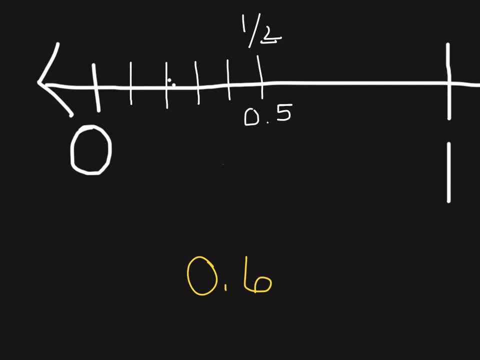 and let's check my work now to see if my lines are correct. I always start from the zero and I hop from there. So this is one tenth, two tenths, three tenths of the line, four tenths and then five tenths. Perfect, I've equally spaced lines. Let's keep going the other way. That should be. 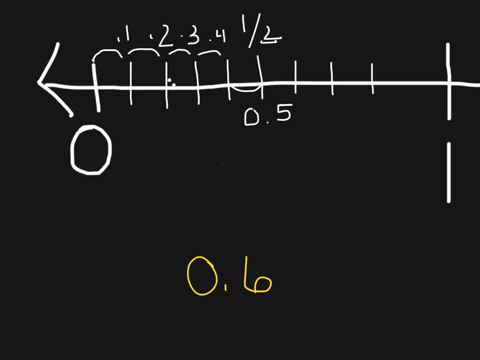 about six tenths, Seven tenths, eight tenths, nine tenths. Let's check my work. That's six tenths, seven tenths. hop over to eight tenths. hop over to nine tenths. hop over to ten tenths. 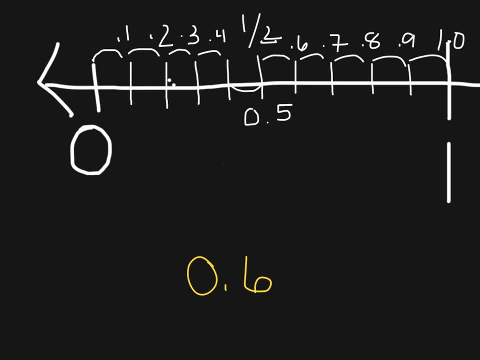 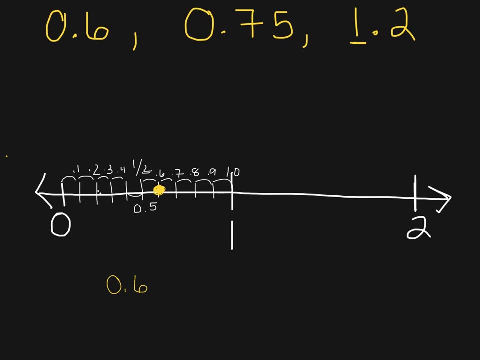 or one whole, Perfect. So six tenths would fall right about here. Perfect, Nice job. Let's zoom back up. Okay, so we have six tenths on our number line, Let's do seventy-five hundredths. So when we say seventy-five hundredths, that means that really we should be placing this number. 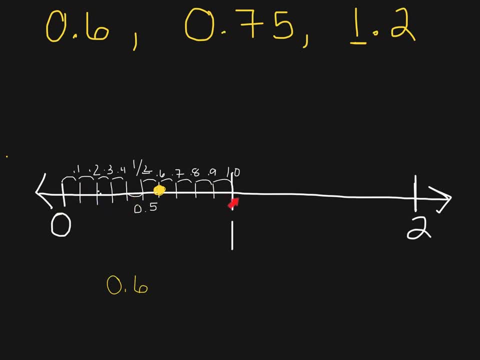 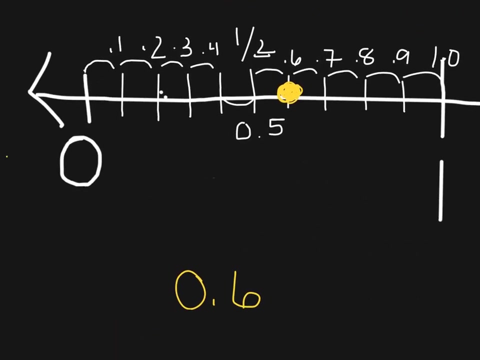 between the zero and one and cutting up this space into one hundred little pieces, because we're working with hundredths. However, that's a lot of work, and let's show how we can simplify this by zooming back in. So we've already cut up our spaces into tenths, which is fine, because we 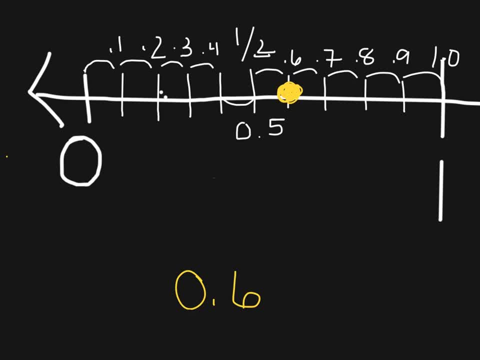 have seventy-five hundredths, meaning a seven in the tenths place. Let me show you what we're going to do here. Let's just write down our number. So we're going to be working with the tenths place here and it's going to be between the tenths place. 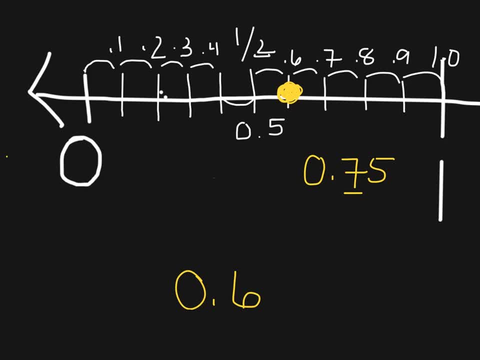 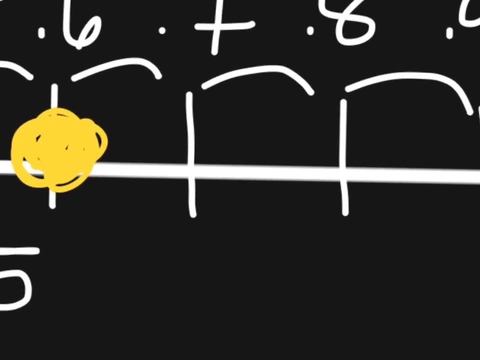 of seven tenths and eight tenths, because there's no eight here but we have a seven. So we're working right in these spaces, right here Now we have a five which tells us it's going to be halfway between the seven tenths and the eight tenths. If you wanted to, you could certainly cut up. 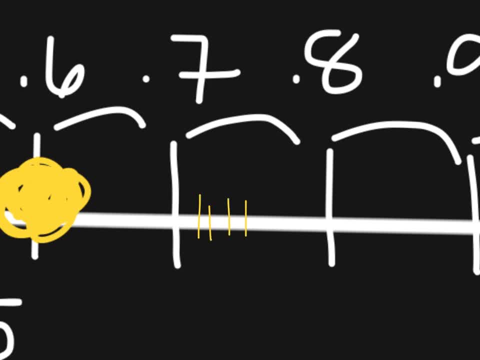 these spaces between the seven tenths and the eight tenths into ten equal spaces. I don't know if I did that correctly. Let's see, That's one, two, three, four, five, six, seven, eight, nine, ten. I did, I got lucky, So this would be seventy-one hundredths, seventy-two hundredths. 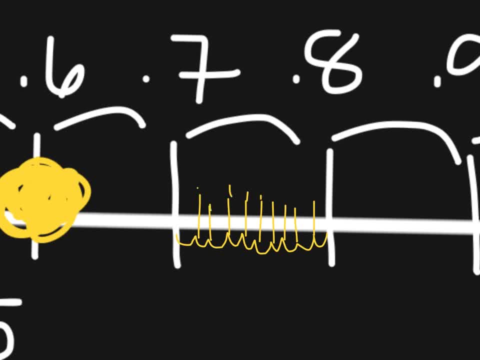 seventy-three hundredths, seventy-four hundredths, seventy-five hundredths, seventy-six, seventy-seven, seventy-eight, seventy-nine. You get the point. So seventy-five hundredths would be right about here. All right, So let's zoom back out and let's do. 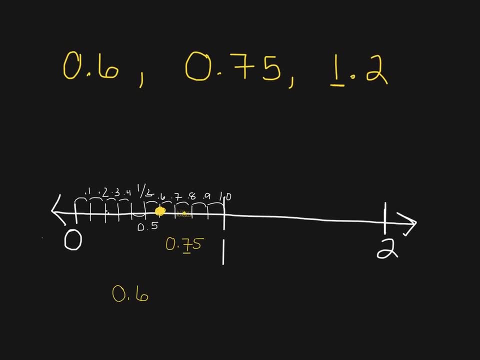 our last number. It's kind of tiny, Sorry for how tiny. that is Okay. One and two tenths, So we're working with a number that is more than one. this time And the same thing, though. We have tenths, meaning that we need ten equal spaces between the one. 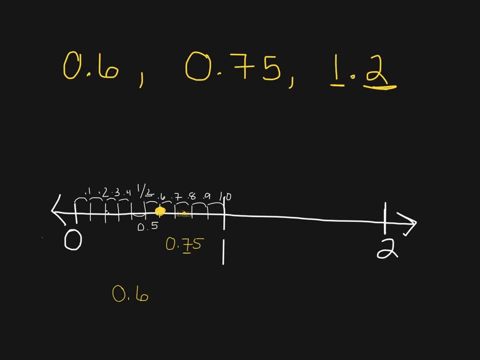 and the two. So since we've already done this, we're going to kind of breeze through it a little bit quicker here. Here's halfway between one and two. So this is not just half, this time It is one and a half. 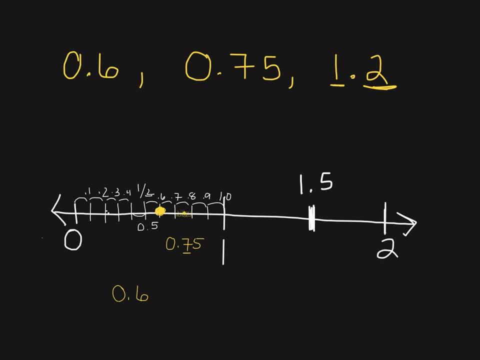 All right, So now we need equal spaces between the one and the one and a half, Or as equal as they can be, And then the one and the half and the two. Okay, So we start from the one, and this would be one point one, one point two, one point three. 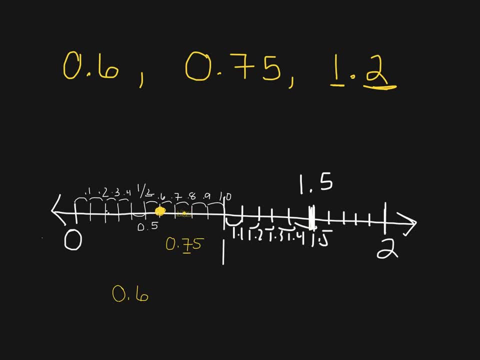 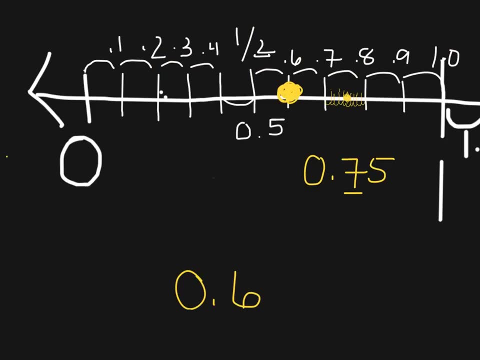 one point four, one point five And our one point two- I'm sorry, One and two tenths is going to be right here. So there you have it. We have this whole set of stuff. So now we have the it. we have placed all three numbers on a number line. Pay attention to that. 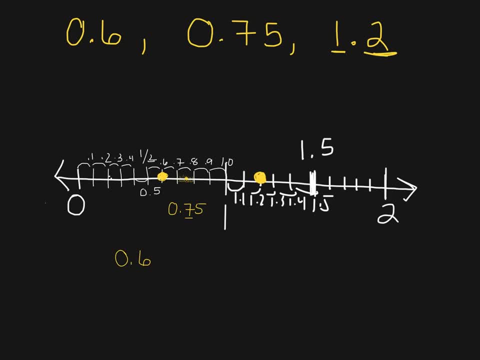 decimal When you say it. that's going to tell you how many pieces you should be cutting up your interval between your whole number. Hope this helped. Watch it again if you need some more assistance, and we'll see you later. 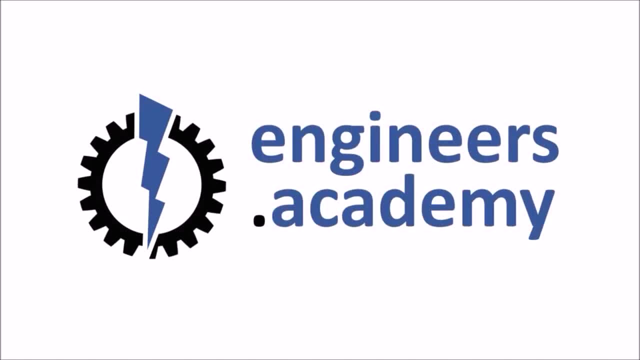 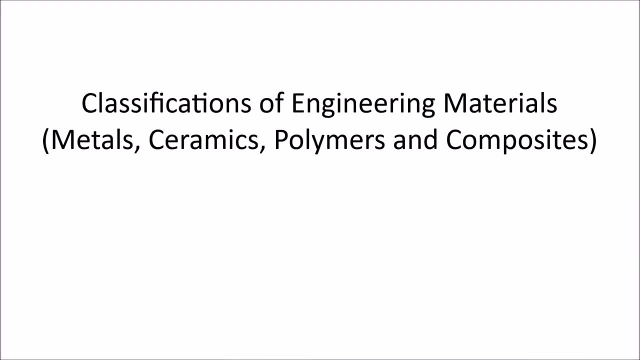 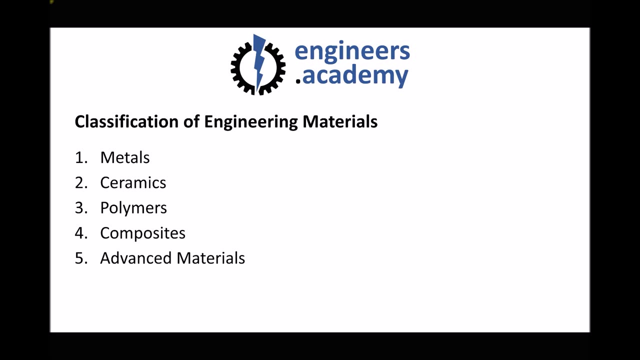 In this video, we're going to introduce five different classifications of engineering materials, and we're going to discuss those briefly, just so that we know how to classify different engineering materials into one of each of these classifications. We're then going to talk about some of the properties that relate to each of these classifications of material. 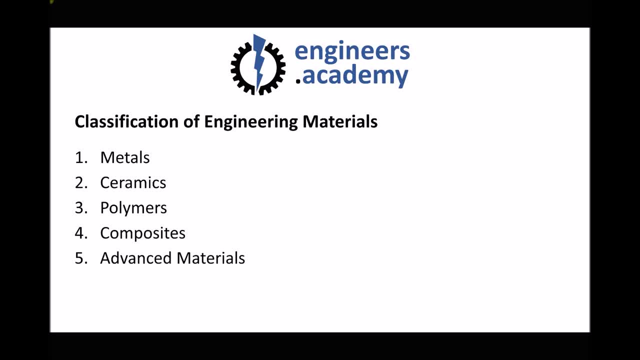 So what we have here is we have five different classes of material. We have metals, ceramics, polymers, composites and advanced materials. Now, for the purpose of this video, we're only going to look at the first four: metals, ceramics, polymers and composites.